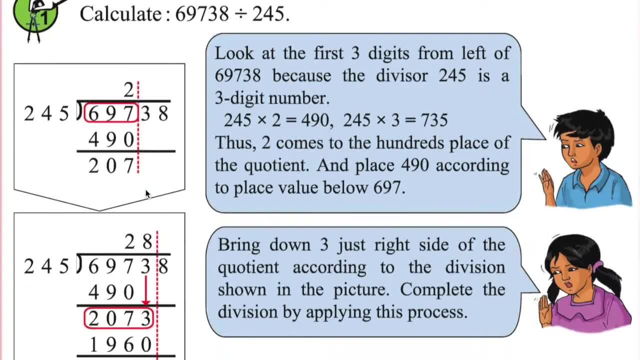 207. after that, you have to take one digit at a time. okay, 3 will come down. okay, 3 will come down. now let's see which number will fit here. okay, since this is 2000, maybe 8. okay, 8. 2. 45 is a 1960. okay, 8, 5 is a 40, 4, 8, 4 is a 32. 6, 3, 8, 2 is a 16 plus 3 is 19. 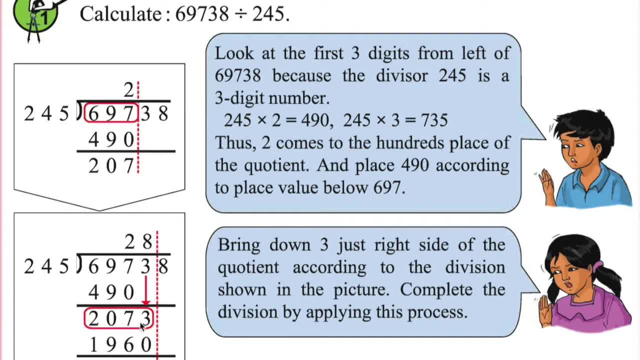 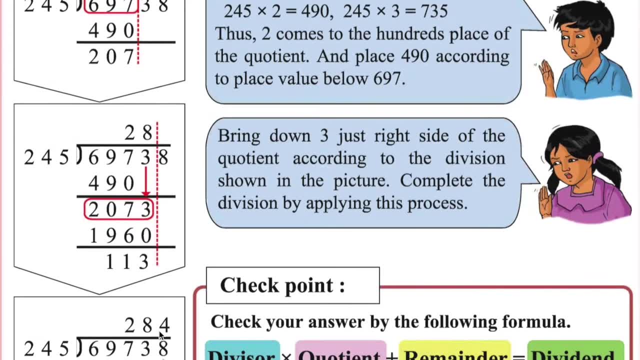 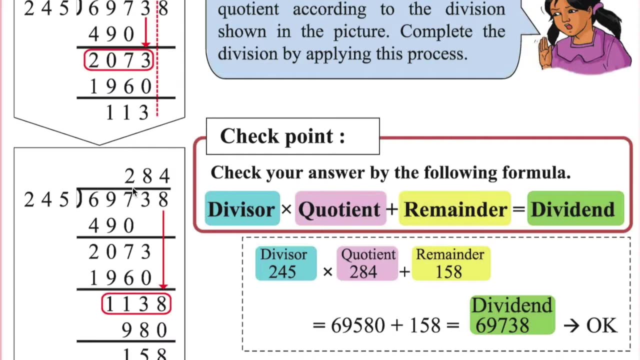 okay, if you go for 9, that will be larger than 2, 0, 7, 3. that is the reason why we took 8. okay, and what is the remainder? 113? now, 8 will come down. okay, let's see which number will fit here again: 4 if we, if you take, if you take 5. 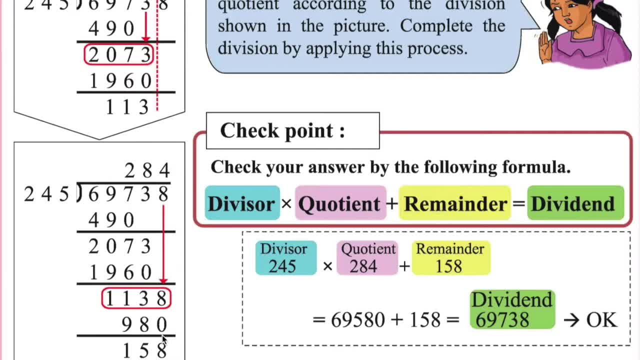 it will be larger than 1138. that is the reason why we took 4. the remainder is 158. 158 is less than 235. always, you remember. you remember that the remainder is always less than divisible. okay, okay, check your answer by the following formula once you found: 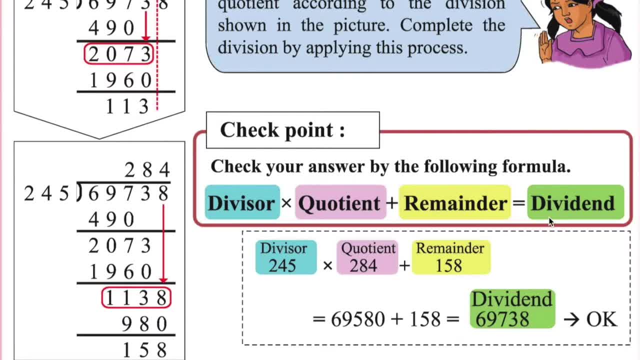 something here you need. you can check the value, whether the obtained value, whether it is correct or not, by using this formula: divisor into quotient, or let's say in to quotient plus remainder, must be equal to the dividend. this one is called dividend. okay, this is divisor: divisor into quotient plus remainder. 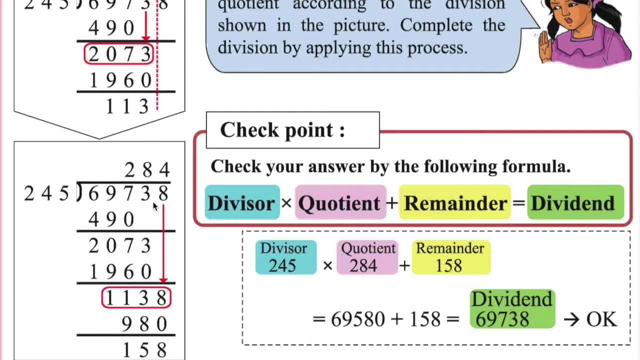 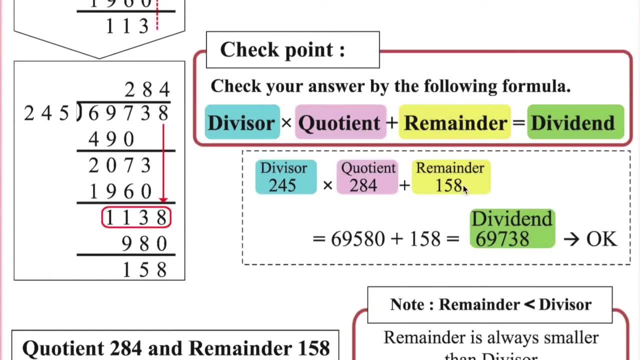 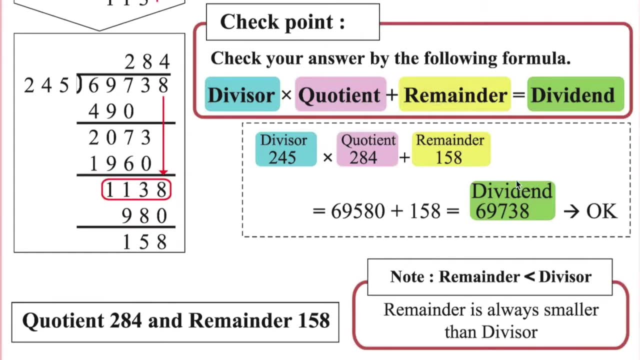 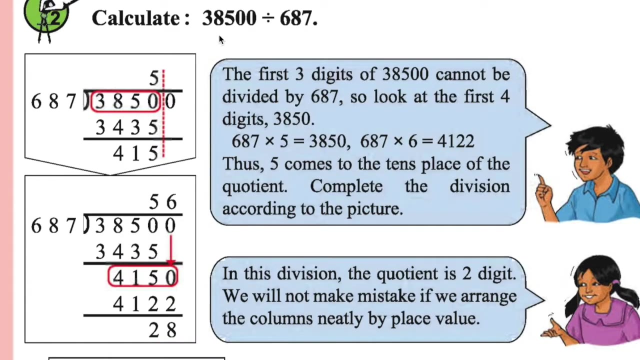 must be equal to the dividender. okay, and always. you remember that the remainder is always less than 20-оты hr is 284, remainder is 158. so when you do this math, simple math, you will get the value as 16738. there is nothing but dividend then this is correct. so this is correct. now we will calculate 38 500 by 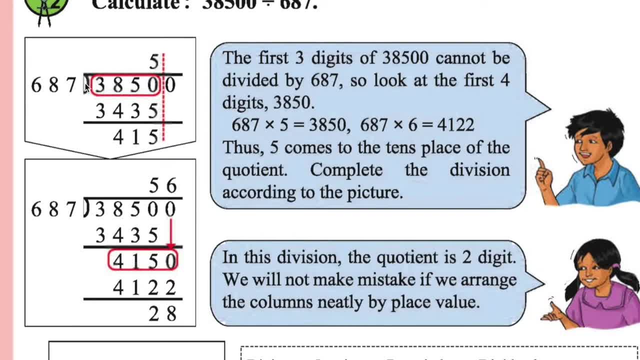 687. again how many numbers you have to take. see, 385 is less than 687. that is the reason why we took four numbers. if the three numbers or more than 687, we would have taken only three numbers. okay, you got the point. you got the idea. now multiply it with five. if you take six, that will 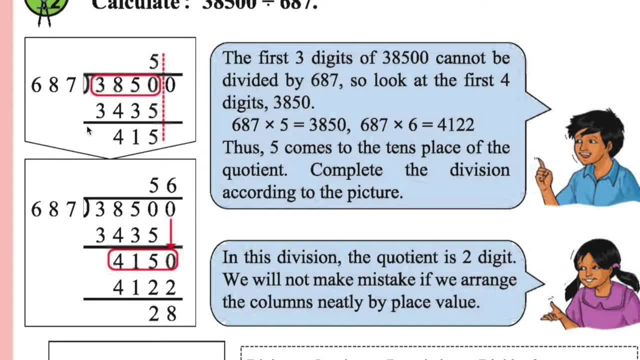 be more than 3850. that is the reason why we took five. this is three, four, three, five or this minus this gives you 415. the this 0 will jump down. okay, now 6 will fit in 4122 and the remainder is 28. 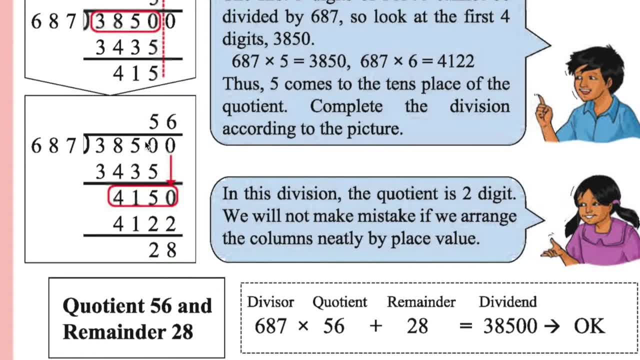 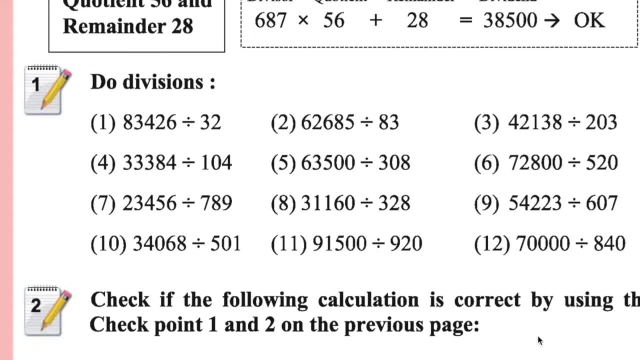 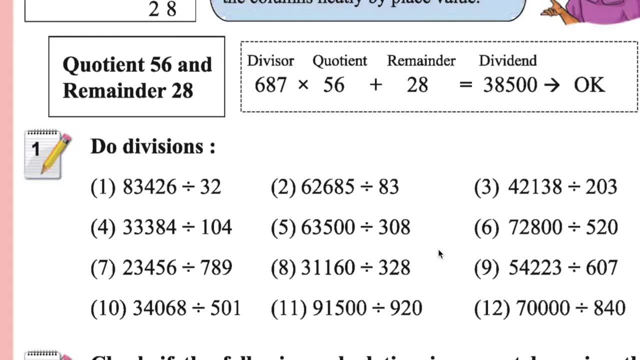 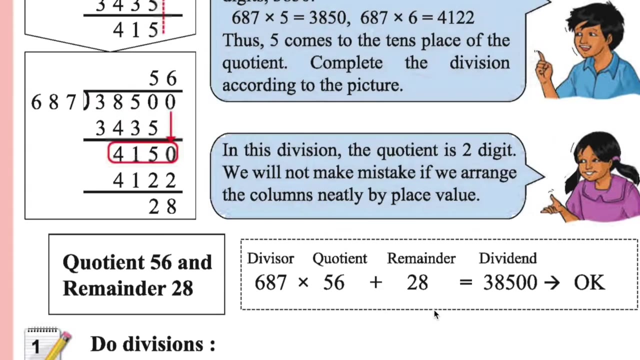 again. you can check, uh, into quotient 687 plus, into 56 plus remainder equal to your dividend: 38 500. okay, now you have to do these divisions. let me show one division at least. where, where, where i can show these divisions? do i have space in the upper? oh no, exercise one, it is. 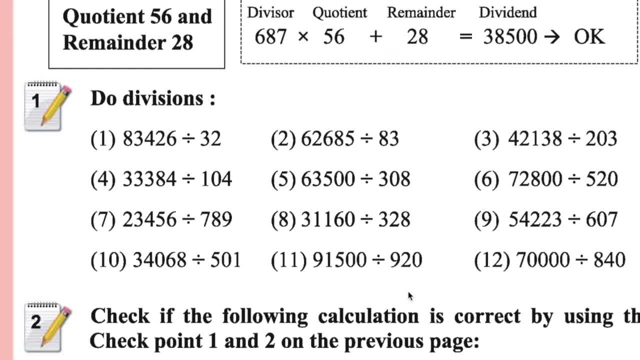 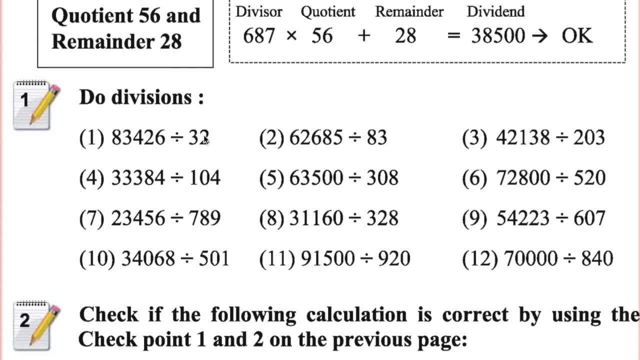 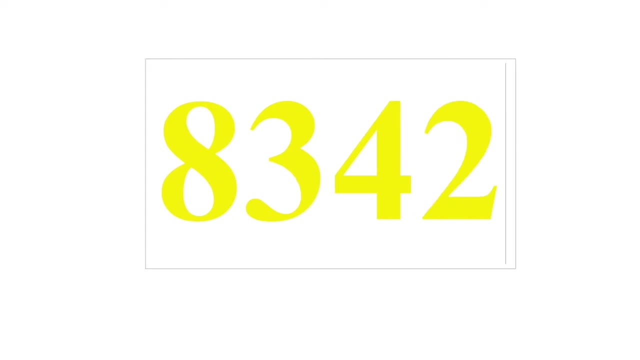 okay, um, okay, i will do one thing. okay, what i am going to do is i will take my extra sheet, because the space is not sufficient. we just need to remember this number: 83 426 divided by 32: 83 426, oh, 83 426 by 32. okay, we will change the color. 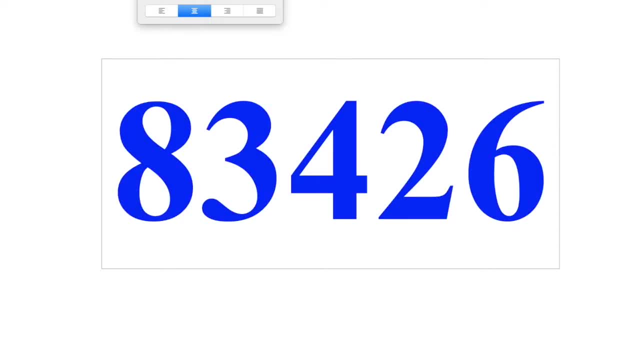 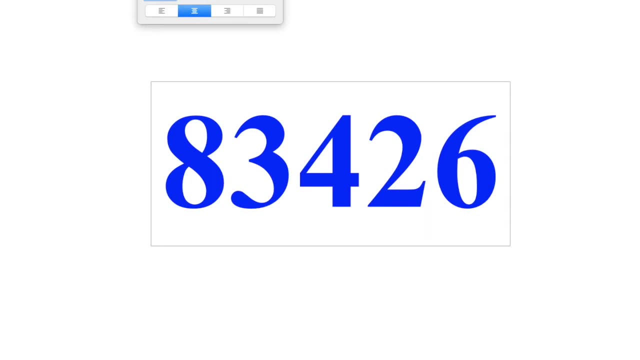 black is fine. you want blue? reduce the size. oh, this is going to take long, long time. okay, that is fine. uh-huh, um. okay, we need what? curved back, the brackets like this. okay, this side also can be cut out, and then also you can see that is also the same um. 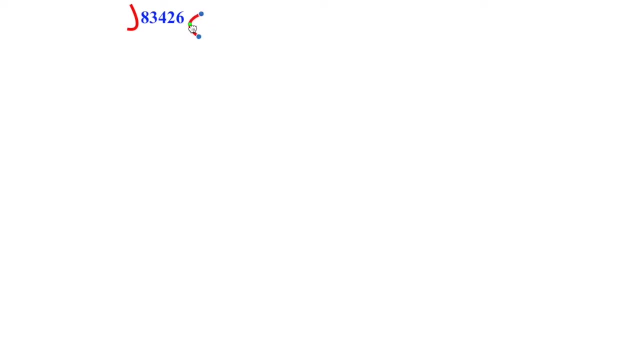 actually, by any means we can talk about this by adding this and so on, and this is where there is this record. we will also take it over to it and this is what we have. we have been supporting. we have taken out this button here for this measurement. okay. 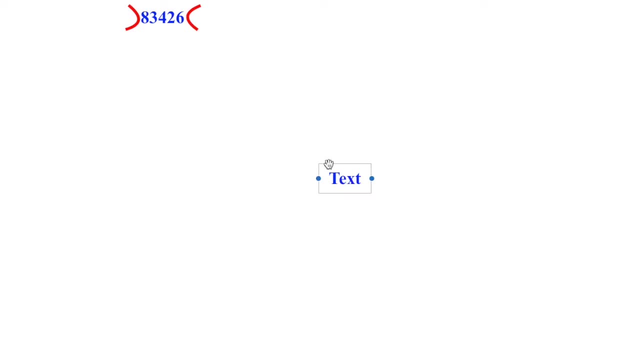 so what we are going to do is we are going to take this function and we are going to call this j RS to j s R. this is the one we were used to- uh j, PS5, Japan, Japan, Japan, Japan, Japan, j to do. we can do that kind of thing, but let's not do by that method. okay, now we will restrain. 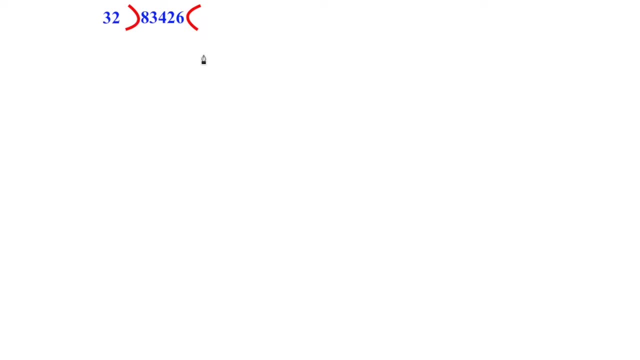 ourselves by not doing, not using any other method than the long division. okay, see, 32 is less than 83, so that is the reason why i took only two numbers now. i'm going to take only two numbers now. uh, 32 to the 64, 32, 3 is more than 83, so that is the reason why i took only two here. 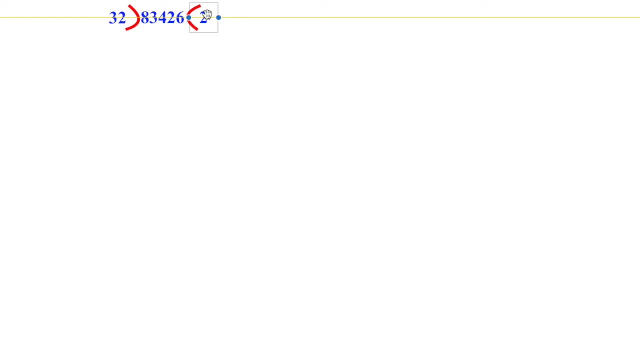 okay, i'm proceeding with two. okay, what is the value? 64. okay, now you need to subtract 64 from 83, draw a line then okay, uh, then what is the left out value? uh, 64, 670, 10, 17. yes, 19, maybe perhaps 19. yes, that is 19. okay again, uh, bring four here. 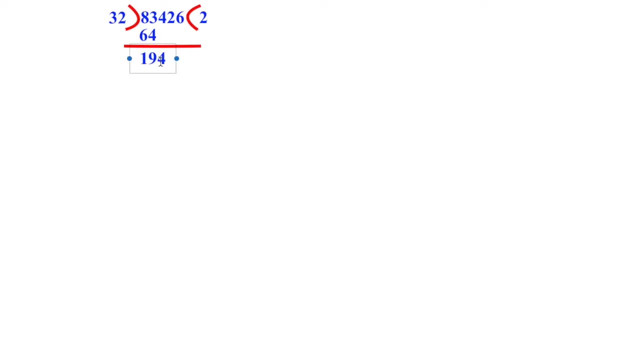 you need to bring. bring one, only one digit from the down down the line. okay, uh, what about this? uh 32, how many times? 4 is 12? uh 5 is 15, 6 is 18.. i'll boring required 6, how much 6? 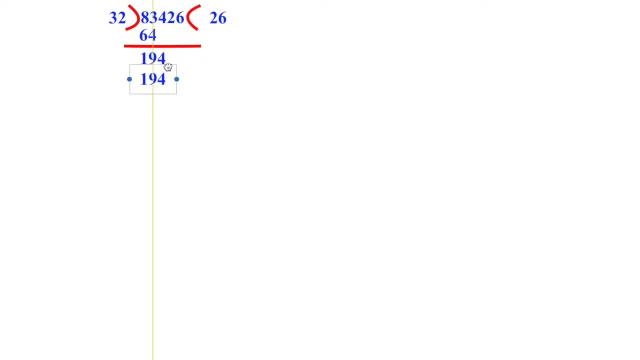 yes, 0.5. what is the value you got? value is not 194, that is 182 square this line right? okay, let's use that. line 2 has to come down. okay, reminder is 2. again one more: 2 is there. that has to come down. see here, 22 is less than 32. how can you? 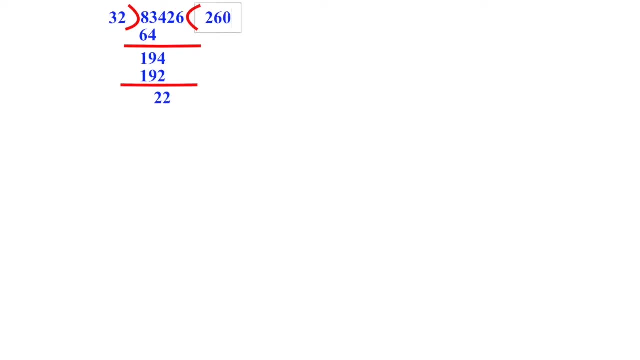 do that. then take 0. with the help of 0 you can bring the 1: 6 down. okay, the other number down just using the using 1: 0. that means the other number will come down: 32. how many times 226? so 32, 6 we just now see is 192, okay. 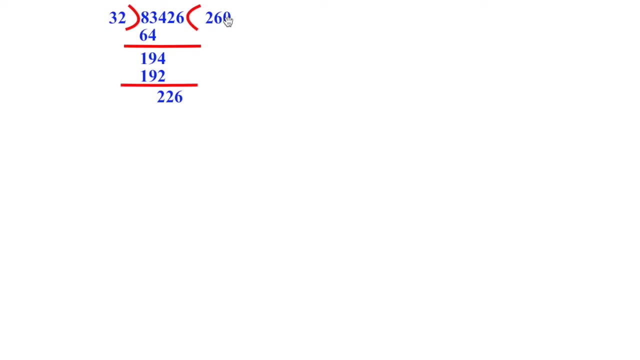 then we will go with 7. yes, 7 will be the correct match. 7, 2 is a 14. 4 has to come first. 7, 3, 2, 21, 22, 224. again, you require this line, then how much it will be the? 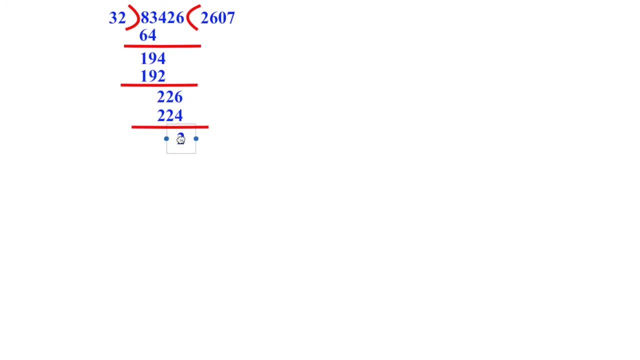 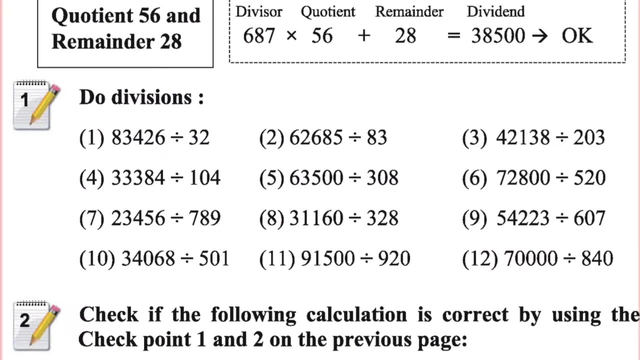 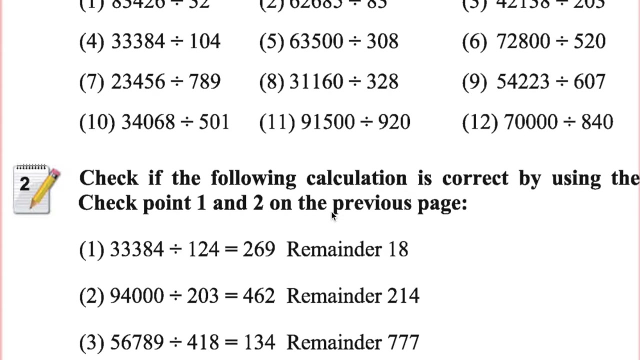 remainder will be 2. okay, so quotient is 2607. now, reminder is 2. what has been asked? do the division. that's it. so you need to find the quotient and the remainder. we found it right. okay, you have to do all the remaining things. remaining divisions: check if the following calculations is correct by: 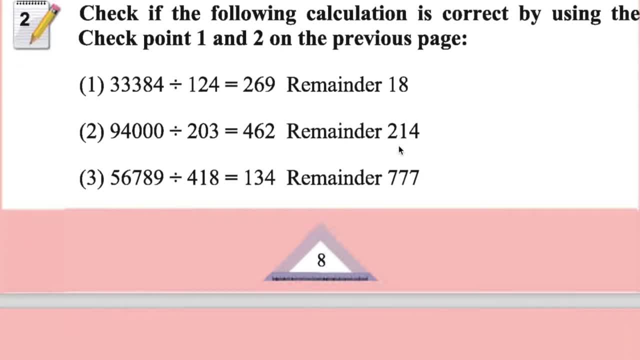 using the checkpoint 1 and 2 of the previous pages. see, we need to check whether this one is correct or not. okay, 124 into 269. okay for remainder, is your remainder 18? then this into this, plus this must be equal to this. okay, so again, what happens? nothing happened. this becomes 120. 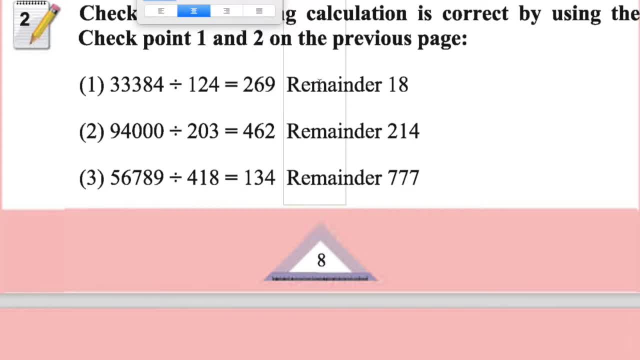 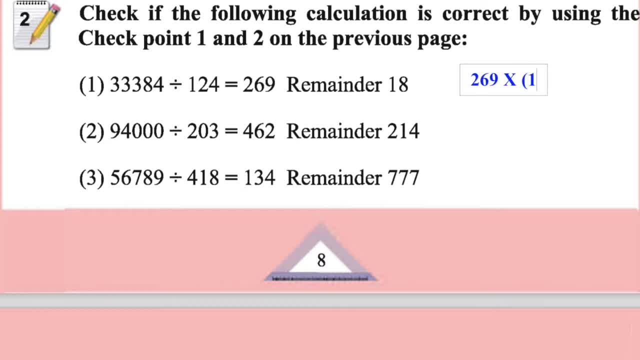 perhaps how this? I can write it as 100 plus 24. equal. to see by multiplying 100 is very easy. just add two zeros or 24. how can I write 269 into 24 can be written as 25 minus one. okay, is that fine? we can equal to 2 6 9 0 0. yes, 2 6 9 0 0 plus. 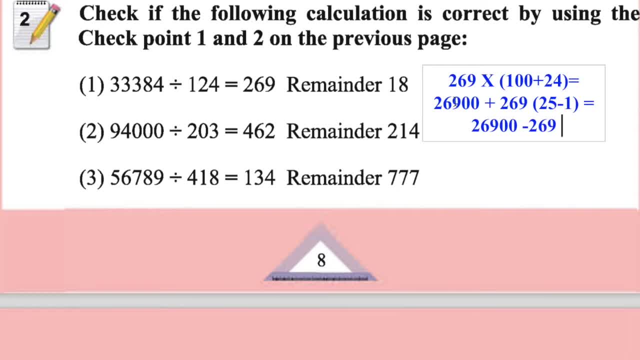 minus 269. last digit I am writing here is this: multiplication plus 265 into 29 instead of 25: 25, 25, 25. I can take it as 100 by 4, right, is that fine? now remove 269 from 26900. okay, how much is? 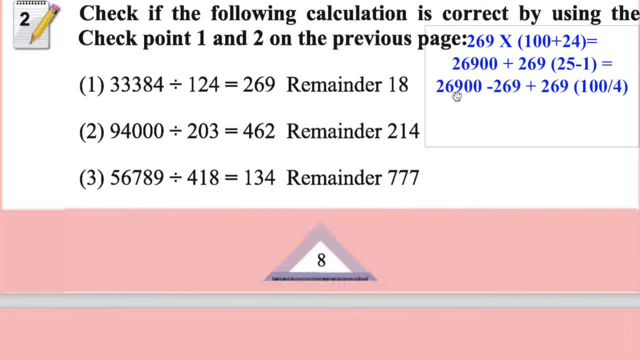 going to be. take 200 from here. okay, from here. if you take 200, it becomes 700. okay, take 60 from here, or 70. if you take 70 from here, it becomes 630. okay, one has to be added right to 26631, and this is 26900 divided by 4. 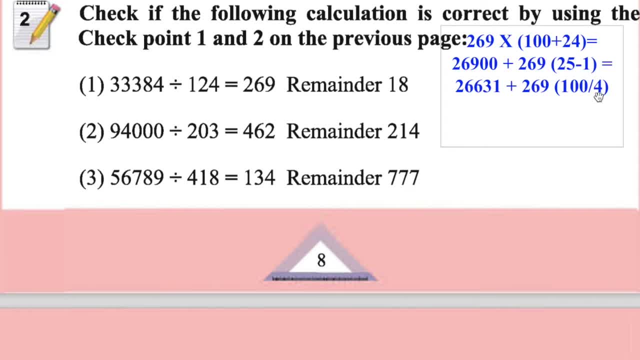 hmm, yes, can we do that easily? yes, it will go by. hmm, it will go by two or four, i guess. so, yes, it will go. why not? last digit is zero, right? so four fours are 24. okay, equal to- i have to write it here- got 26631 plus for for the 24: 00. 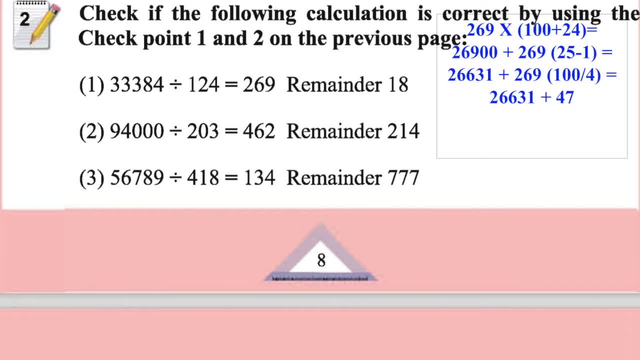 4728 mm-hmm. 4208 mm-hmm. 40420. is that correct? in support later on: deeper 2j: 10, 1, 4, 7, 0, 28 point 1, 2, 4, 4, 0, 24 plus 2, 26. that is correct, no problem, now we are. 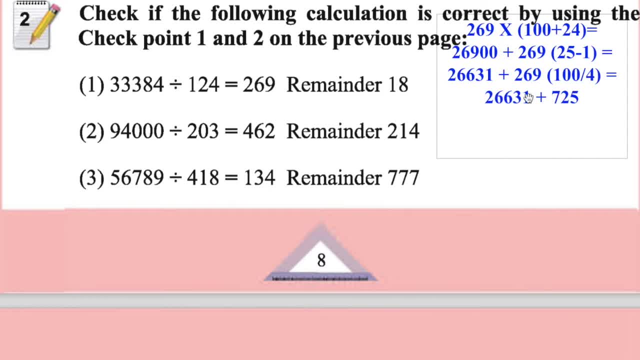 going to add a 4,000 first to 26. we had 4,000 here, this becomes 30,000, okay. now. I had 25 at 700 first, 700. here. three, three need. this leads to three, three, okay. 20 here. then this becomes 51, okay. lastly. 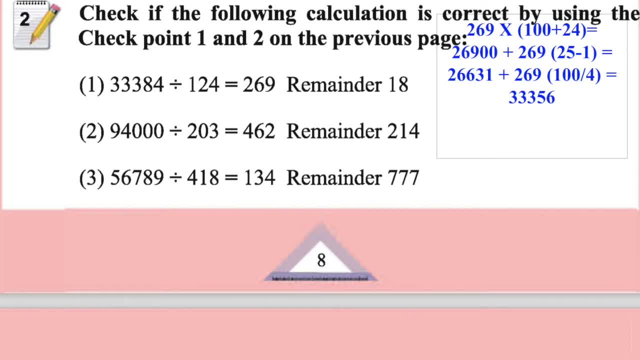 five, this becomes six. okay, now add 18. if we add 18 to this result: three, three, three, 5, 6 plus 18, 8, 6, 0, 14, 4, 1, 5 plus 6, 0, 5 plus 6, 7, 3, 3. oh sorry, this must be 3, 3, 3. 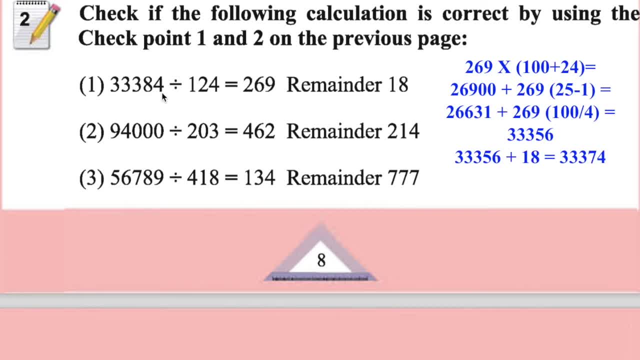 is 7: 4 not 8: 4, okay, so that is the problem. actually, we need to check it quite carefully, okay, otherwise your errors may arise. okay, if you want to cross check here, you can cross check it, I have no objection. but but what I am going to say is, if you do this simple thing to 69 into 124, let's. 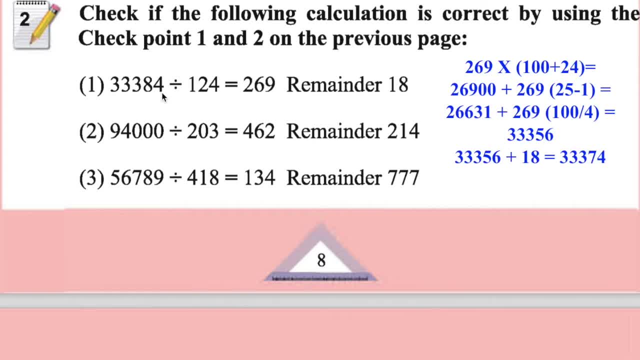 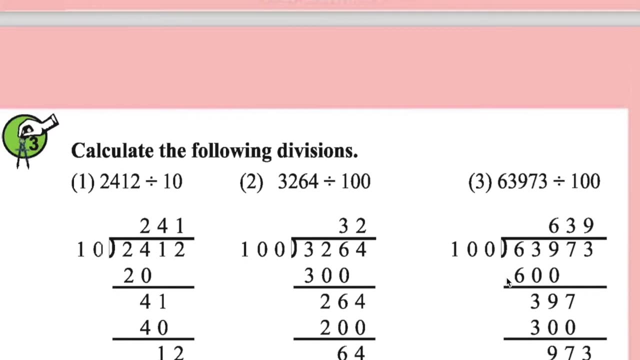 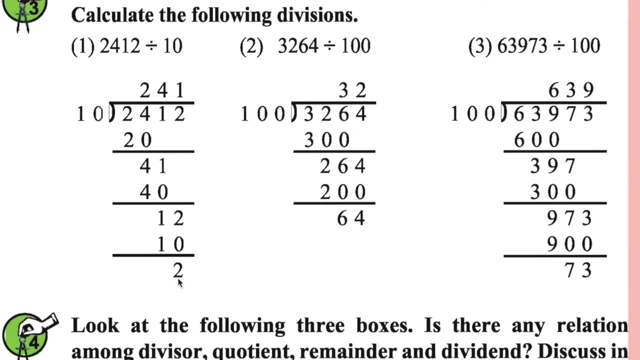 say 10. yes, what we did is quite correct, so much like the following characteristics is correct or not? that is what he said. this is wrong, okay. similarly, you can check the other things, okay, whether they're correct or wrong. quandary the following divisions: 241.2 or otherwise, 240, 2 as the remainder, whatever the x this. 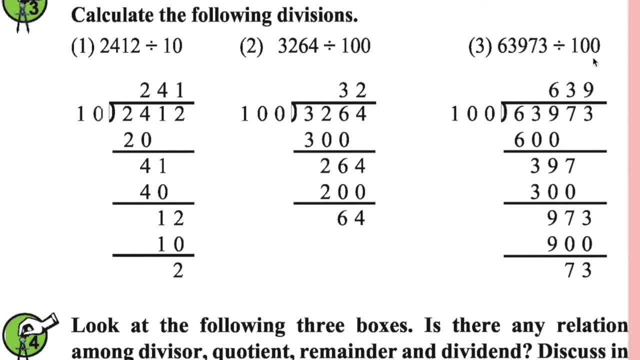 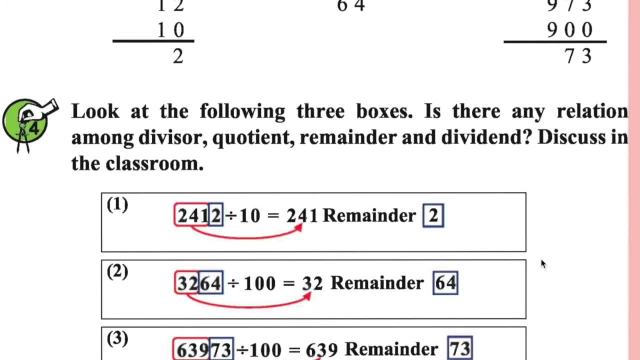 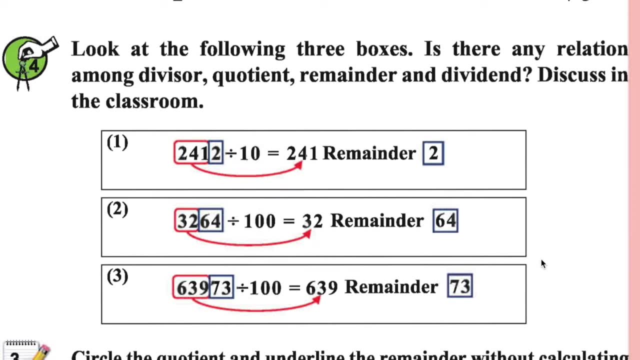 32, 3200, 64 as the remainder. we will get here 639, 73 as the remainder. okay, this, this one, is quite easy when you do the division by 10 or 100. okay, the division is quite easy. see 241. by looking at the numbers you can check how much you will get the coefficient and 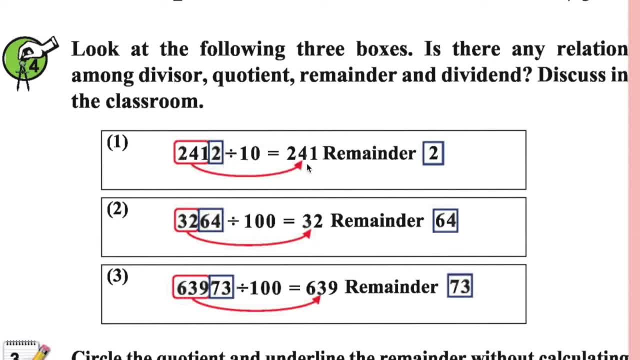 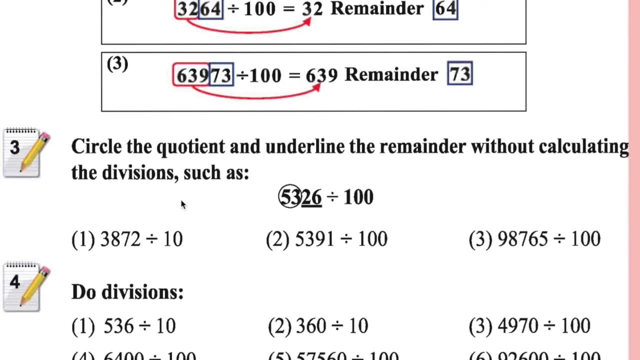 how much remainder. you will get 241 as the coefficient remainder. the last digit, 2, 100, means you will get two digits okay as the remainder and these two as the quotient. okay here also 73 as the remainder. 639 is the quotient circle the quotient and underline the remainder without calculating the divisions. yes, this is the. 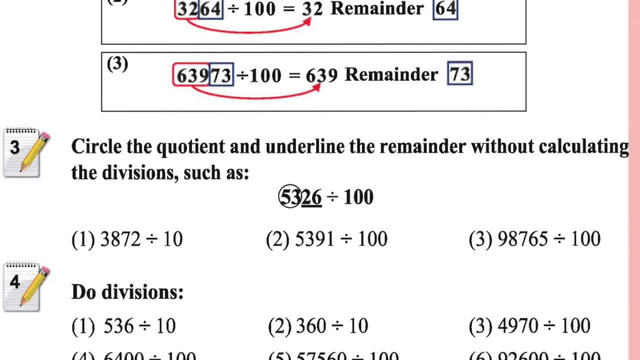 remainder. this is the quotient. likewise, you can, we do the for the rest of the things. yes, that is quite easy. okay, yes, this is what quotient. okay, what about the remainder? you can ask me: what about the remainder? i am going to underline it. okay, yes, okay, oh, no. well, let's uh circulate first. first, let's make that underline part. 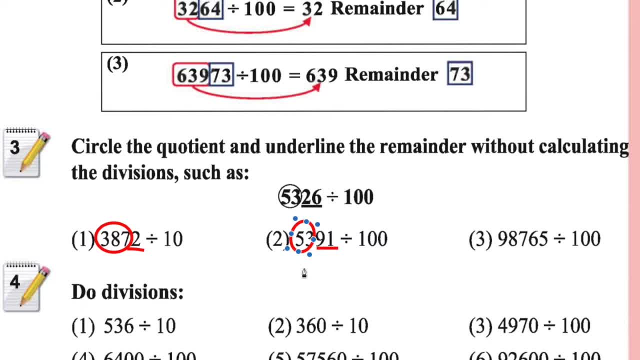 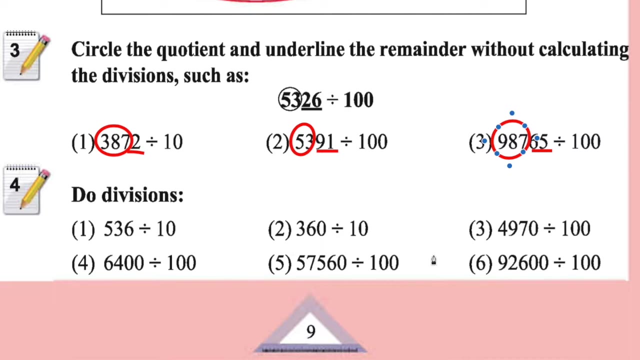 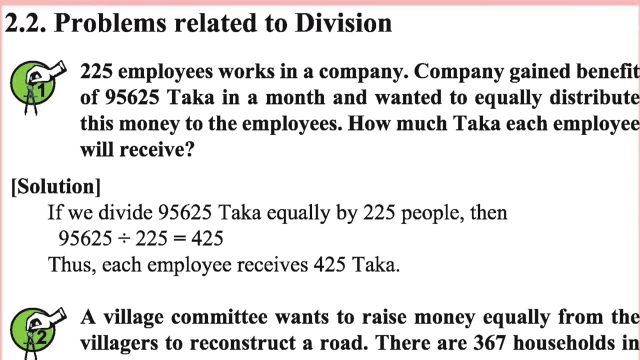 then now you can easily select it. it's quite simple. okay, so now again circle. uh, no, underline the remainder circle. the complaint: okay, all models do divisions. you know the same thing. like similar things, you can proceed in the same way. problems related to division: 225年前 is working a company company gained a benefit. 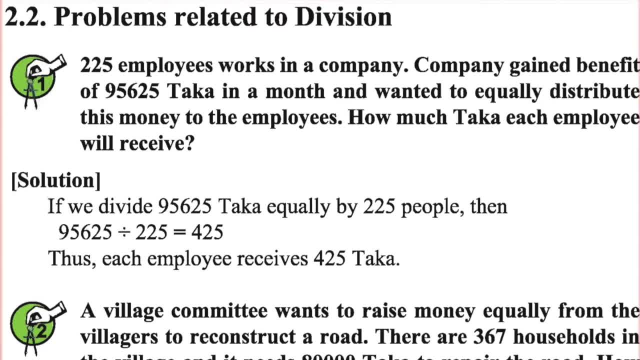 five thousand six twenty five taka in a month and wanted to equally distribute this money to the employees. how much taka each employee will receive? okay, if you divide ninety five thousand six twenty five by two twenty five, you will get a four twenty five. so everyone receives 425 taka. 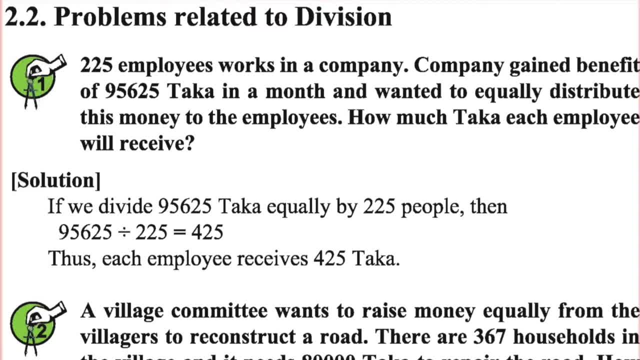 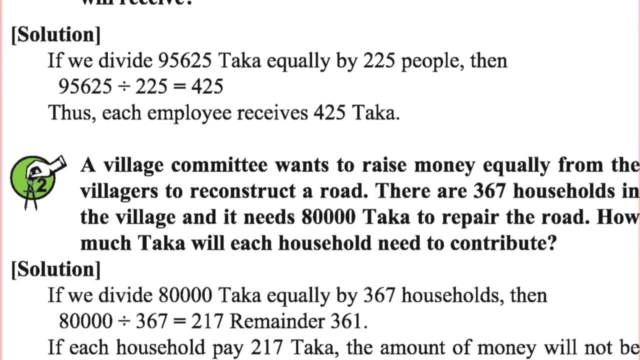 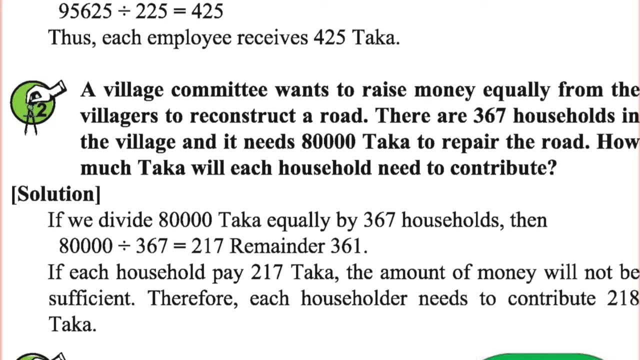 okay, village committee wants to raise money equally from the villages to reconstruct your house. there are 367 households in the village and it needs 80 000 taka to repair the road. how much taka will need for each household? need to contribute 80 000 by 367. 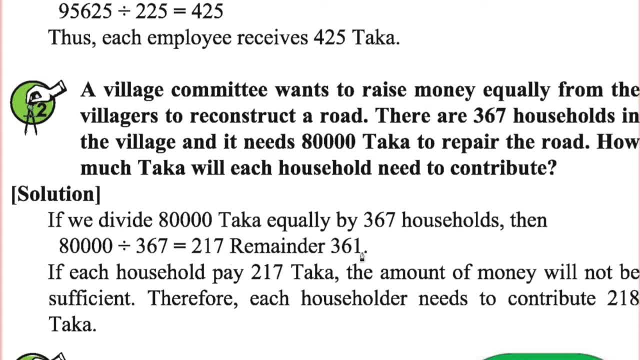 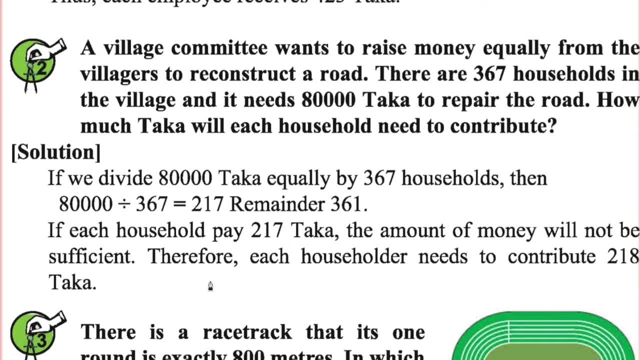 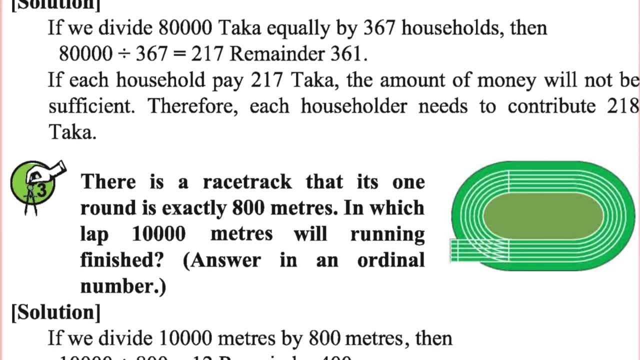 now. then you will get 217 as the quotient, remainder as 361. so if each household pay 217 taka, the amount money money will not be sufficient. therefore, each household needs to contribute 1 rupee more, 1 taka more. that is 218 taka. okay, there is a race track that it's one round is. 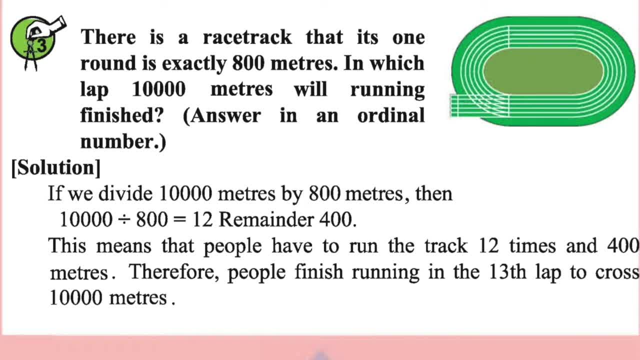 exactly 800 meter, in which lap 10 000 meters will running. finished answering an ordinal number. okay, so if you divide uh 10 000 meters by 800 meters, then uh, you'll get 12, remainder as 400. this means that people have to run the track 12 times and 400 meters. 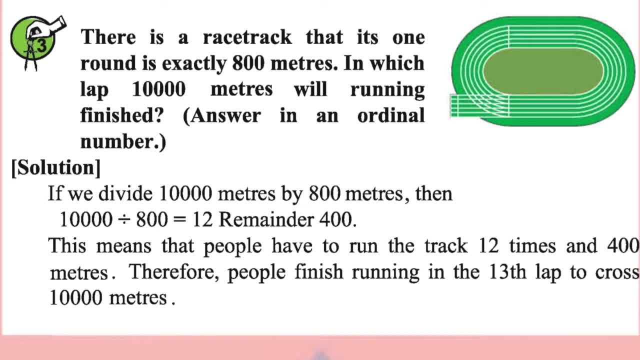 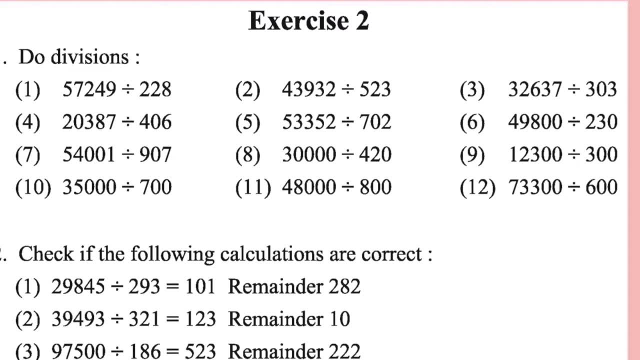 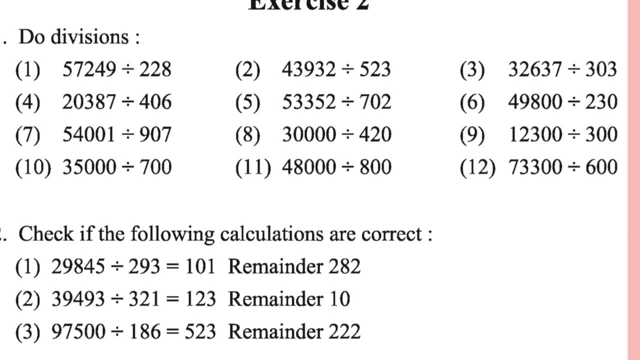 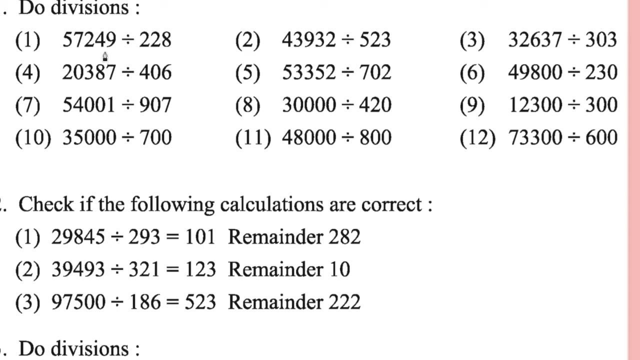 therefore, people finish running in the 13th lap to cross the 10 000 meters. now let's see the exercise to do the divisions. okay, do the divisions fair enough? right, should we do it, because this is three digit. let's proceed. five, seven, two, four, nine, two, twenty. 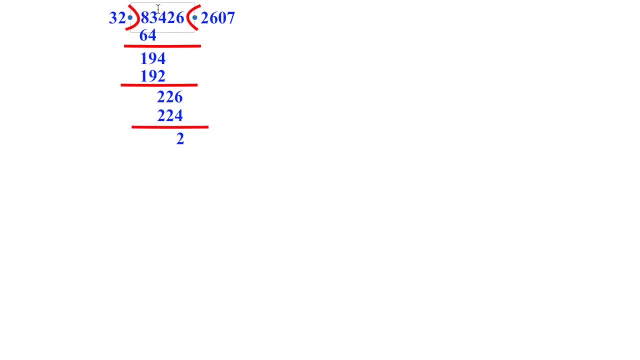 eight, five, seven, two, four, nine, nine, seven, two, four, nine. okay, okay, okay, ok, how much? it is? 229. i think that is 229, 228, 5749, 228, ok, ok, first which digit we have to take? take only first: 3, 228 is 2ja 2868 in 1, 2, 2ja 4, 5, 2, 2ja 4. here 2 will go, 3 will. 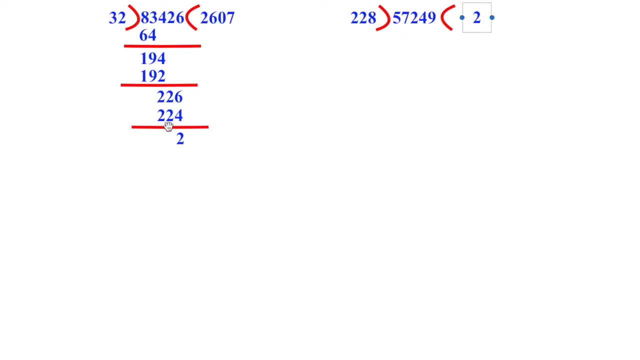 not fit, because 3 2 2ja 6. that means more than the required number. so that is the reason why we took 2 2868 in: 1 2 2ja 4, 5 2 2ja 4, so that is 456, right, we need this line. i saw. 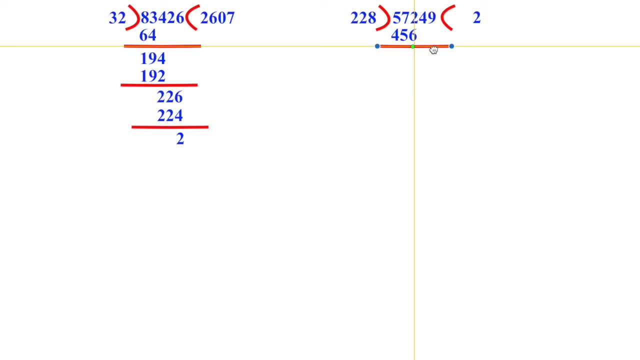 suppose yes, then take this line ok. ok, let's subtract 10-6: 12-6 is 6, 6-5 is 1, 5-4 is 1. again, you need to bring that 4 also down, 4 down, 1164. 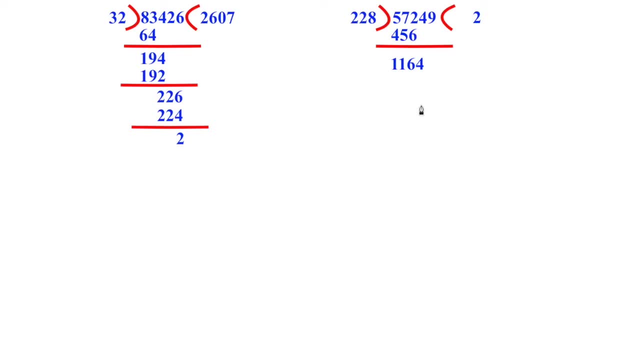 how much it will go? 6, it won't take 5. i think i suppose 5 will. is fine. yes, 5 is fine, so let's take 5. ok, what about the number 5? 8 is a 40: 0, 4, 5, 2ja 10, 1, 1, 5, 2ja 10, 1, 11, 10. 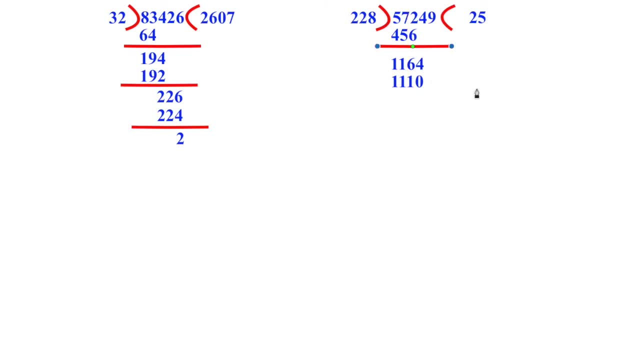 ok, right, we may be requiring that line again. right, fair enough. 64-10 is 54. 9 has to come down, so this is 549, 228, 3ja. it won't go like i said earlier. this will go by 2. only what is what is 228 into 2, 4, 2, 2ja, 4, 5, 2ja, 4, 5, 2ja 5? 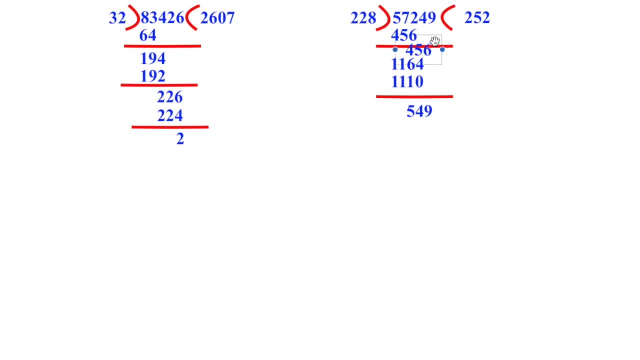 9 has to come down. so this is 549, 228, 3ja. it won't go. like i said earlier, this will go: 456, that is readily available. okay, again, we require this line. take this line, place it here. let's subtract 456 from 549. or let's say, suppose it is 550, if it is 550, 550-450. 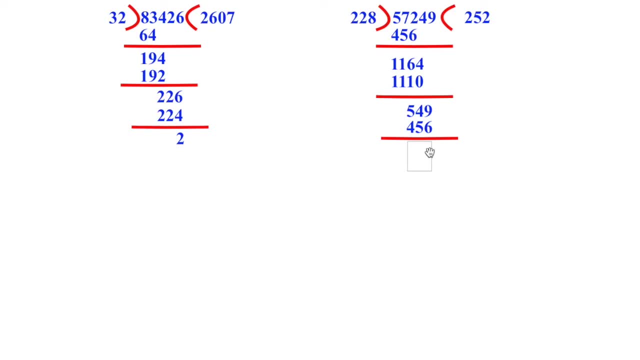 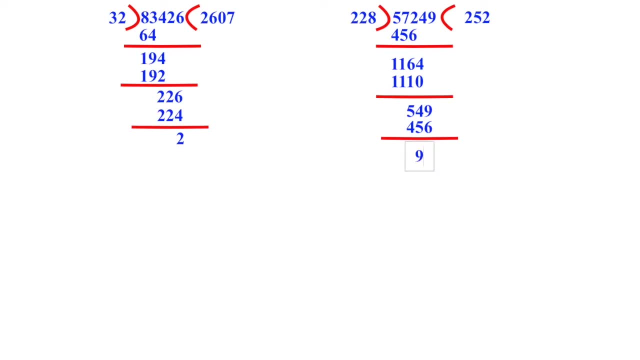 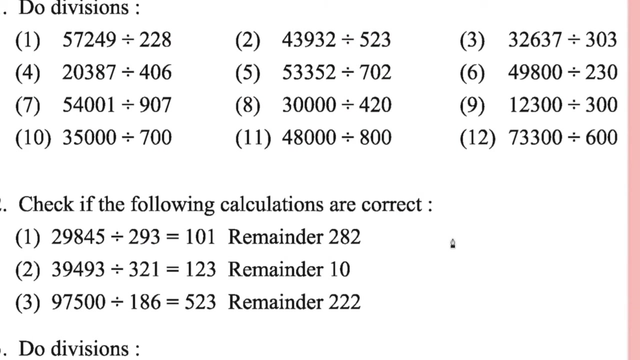 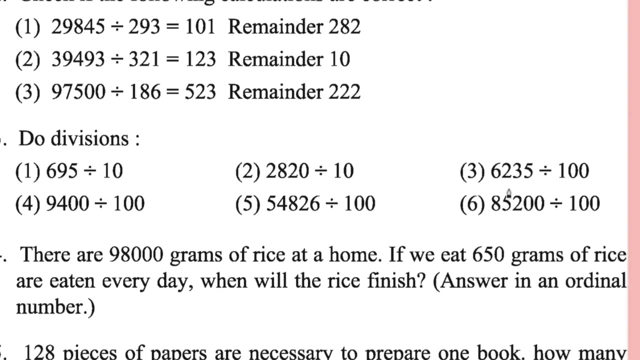 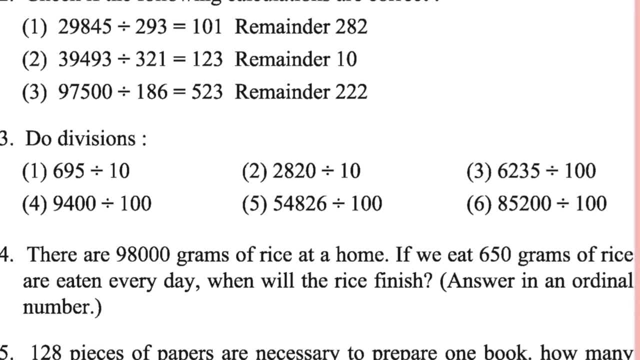 790. oh, they are correct or wrong. okay, mm-hmm, this I am going to check now. all right, first one. I am going to say quite easy: perhaps 293 into 101. I have to do it first, then I have to check with the remainder. how can I write it as 101? I? 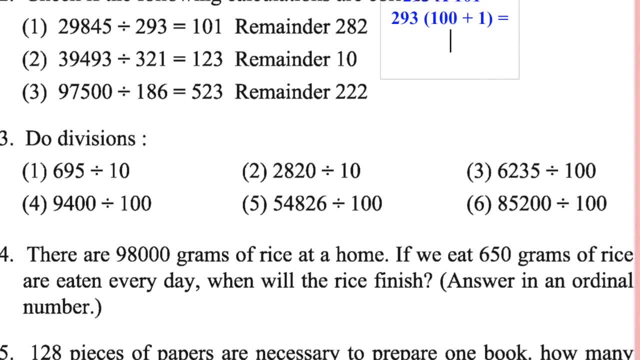 can write it as 100 plus 1, okay, so it is going to be 293 0, 0 plus 293, right, right, then how I'm going to add this number to this? first add 200, then this becomes 500. 200 will vanish. 93 will come directly. okay, so this is the number we. 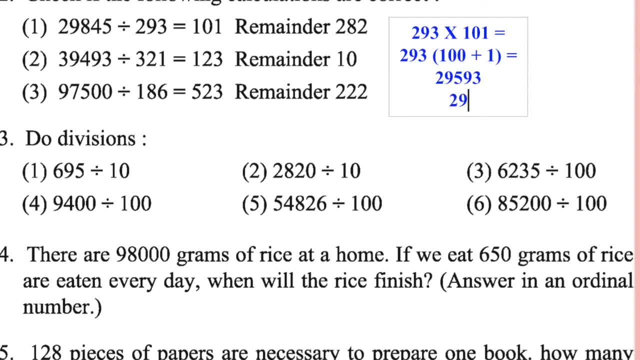 got in the oh, oh the multiplication to 5 to 95, 93. now we are going to add 282 here. to it first add 200. if I had 200 here, it becomes 7, so 2 will go. now add 2, this becomes 80. 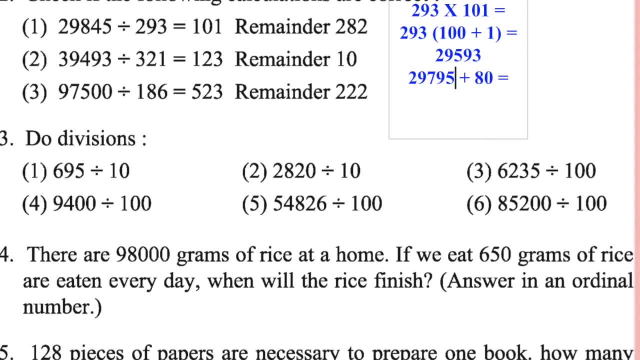 this becomes 5. okay, you are 5 then, Are you serious? Yes, I am serious. This becomes 75.. This becomes 8.. Control: Okay, Now remove these two zeros: 2, 9, 8, 7, 5.. So that is incorrect. Okay, That is how we have to check the values, Okay. 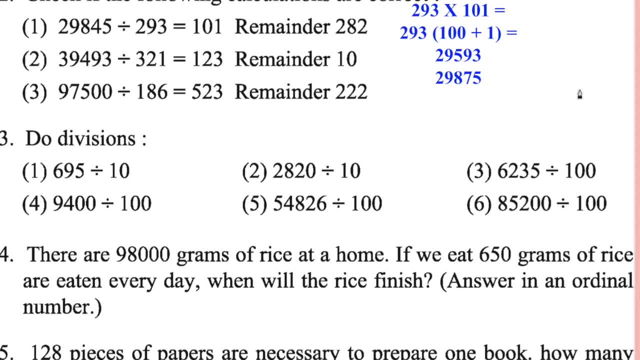 Not quite difficult, But it takes time. That is the problem with the checking. Okay, But anyway, that one is wrong. It is not 845.. It is 875.. Okay, You check with 9,, 8, 2.. Do the revisions. 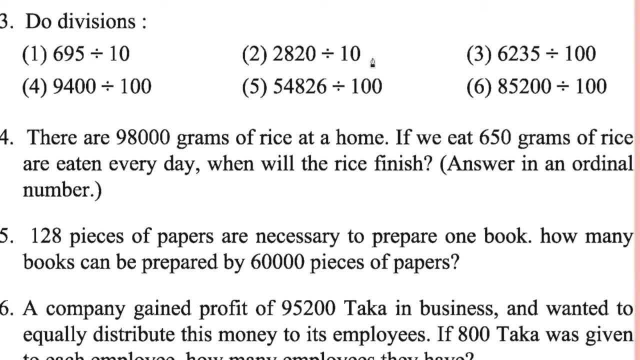 So 69 is the coefficient 5 as the remainder. 282 as the coefficient, No remainder. 62 as the coefficient 35 as the remainder. 94 is the coefficient 0, remainder 548 as the coefficient 26 as the remainder. 852 is the coefficient And no remainder. 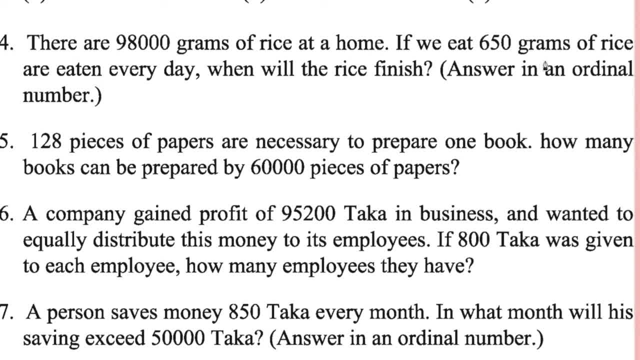 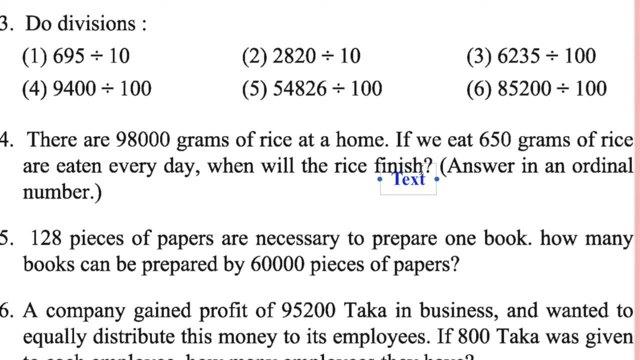 There are 98000 grams of rice at home. If we eat 650 grams of rice at heat and every day, when will the rice finish? Oh, it is not a difficult problem. Okay, Let me get some space here. 98000 divided by 650.. Right, First cut the first zero: 9805 by 65.. That is the problem, Right. 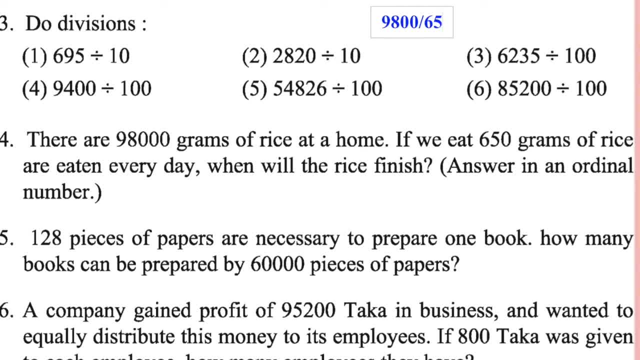 Right Now I am going to multiply both with the 2.. See here: 2, 0, 0.. 2, 8, 16.. 1. 2, 9, 18.. Plus 1, 19.. 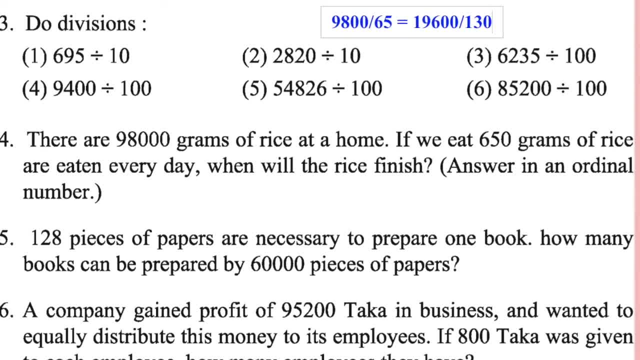 98.. 2 is 196.. Right, So this becomes 130.. Yes Again, 0, 0 will go away. 0, 0 will go away here. Yes, By 13.. Will it go by 13.? Let's see 13,. 1 is 13.. 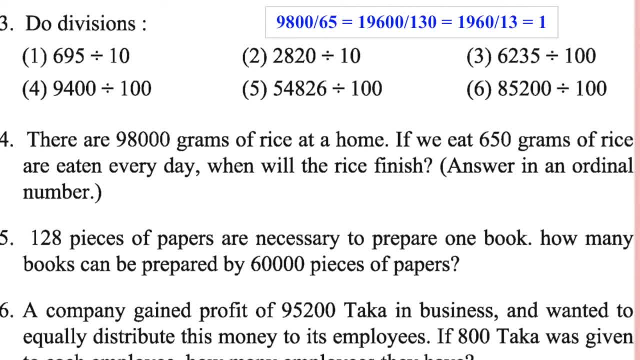 Aha, 13, 1 is 13.. That is correct. 66.. 13, 5 is 65.. Okay, 13, 5 is 65, only Not 66.. that is 1, 15 course and 10 remainder. 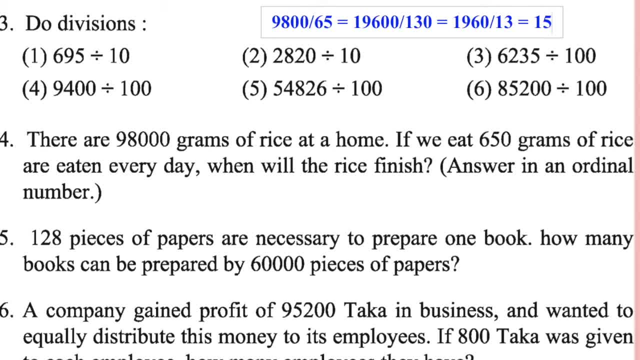 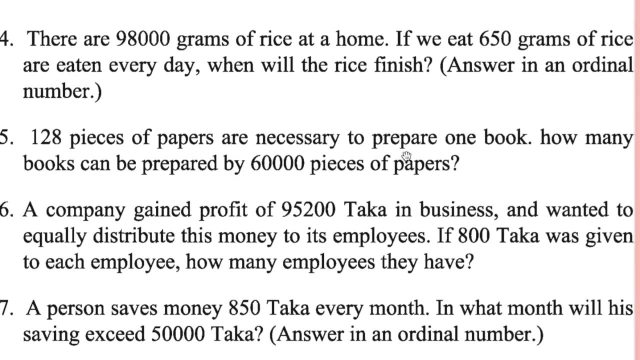 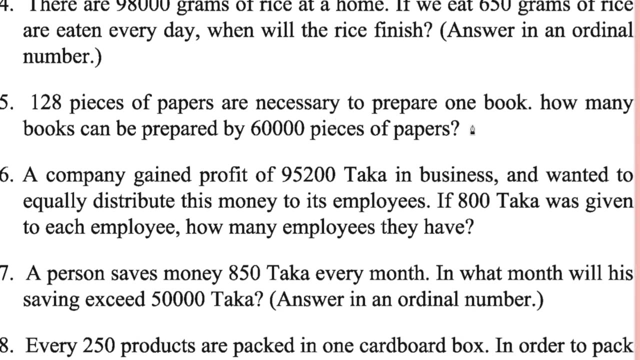 15 days it will finish. 10 grams will be quite less, so I am going to end it here. 15 days, only 16th day with 10 grams. how can you cook so 128 pieces of paper are necessary to prepare one book? how many books can be prepared by 60,000 pieces of paper? 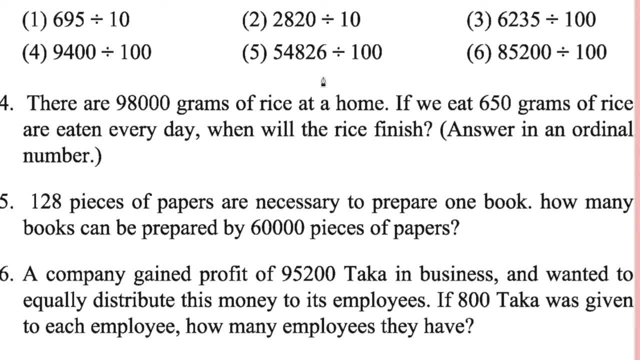 now again, we have to take the 60,000 here: 6, 0, 0, 60,000 divided by 128 pieces of paper, 128, 8. this will go over. it will go over 8. so 8 of 5 is 40. 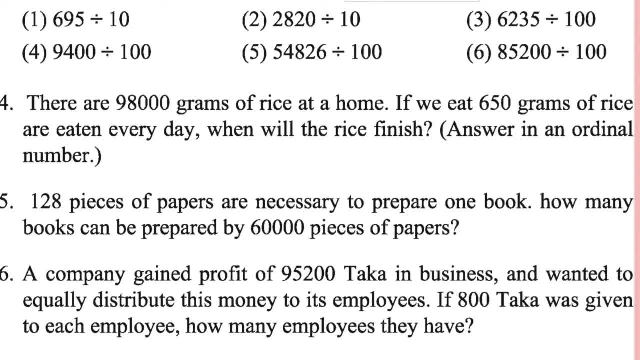 8 of 6 is 48. 8 of 7 is 56. okay, 856. 4, 8, 5 of 40. 0, 0, okay, 8, 1, 8. uh-huh 8, 1, 8, 8, 6 of 48. okay, again, it will go by four, uh, four ones of four. okay. 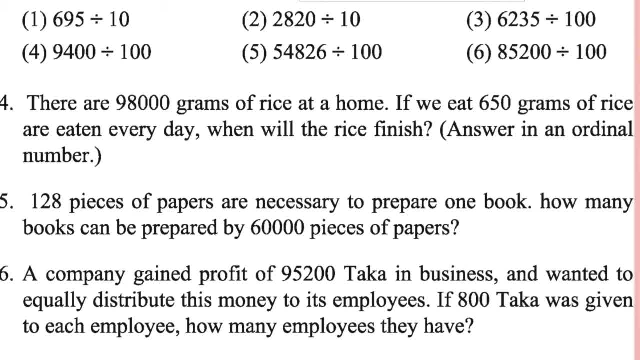 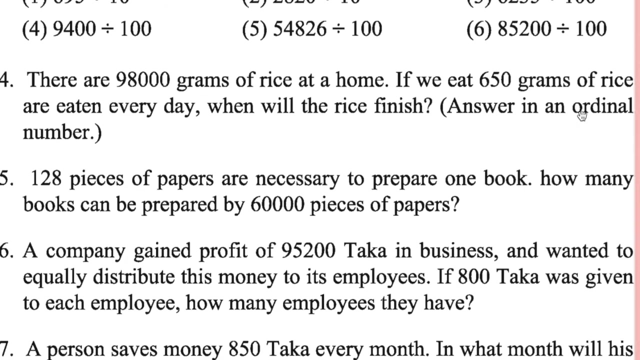 four eights of 32, all right. four sevens of 28, fair enough. four fives of 20.. 1875 by four, okay, now do it four, four, four, job 16, two, four, six or 24 for age of 32, and three by four. so four, sixty eight books only will can can be repaired. 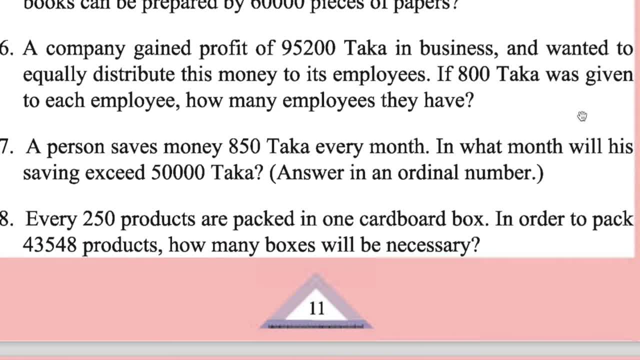 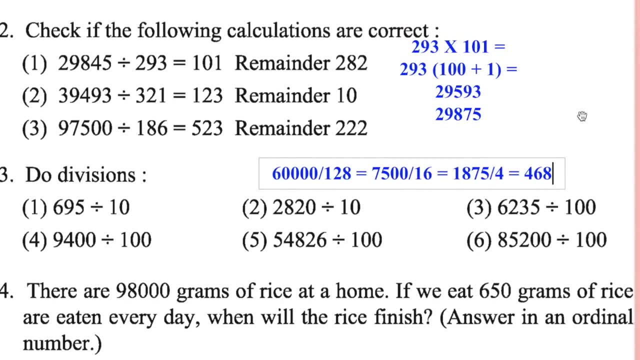 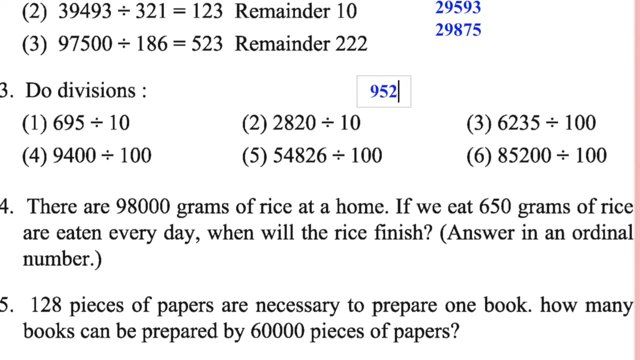 okay, the company gained profit of 95 200 taka in business and wanted to equally distribute this money to its employees. if 800 taka was given to each employee, how many employees they have? so 95 200 by 800, 95 200 by 800: 0: 0. there are two zeros here, two zeros there. we can um cancel them easy, like right. 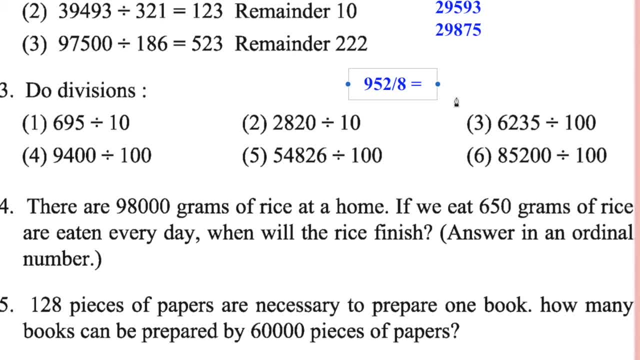 right, so we'll go. will it go away? for i think so. four, twos are eight. one four three is a 12. three, four ages 32 by two. is that correct? four ages 32. three four three. the 12 15, one is two, ones are two. two ones are two. 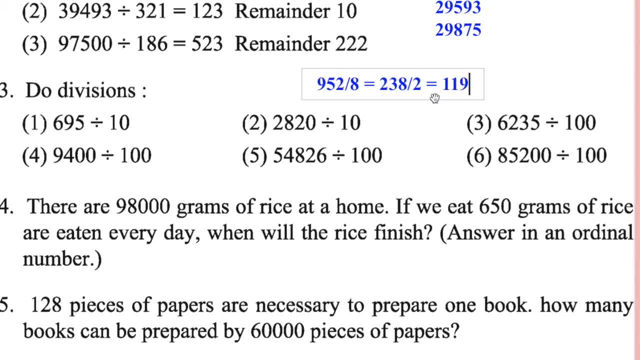 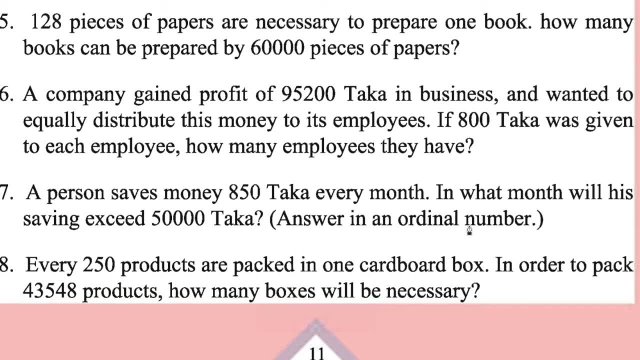 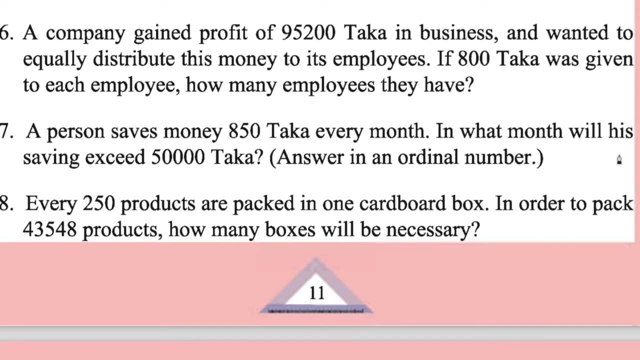 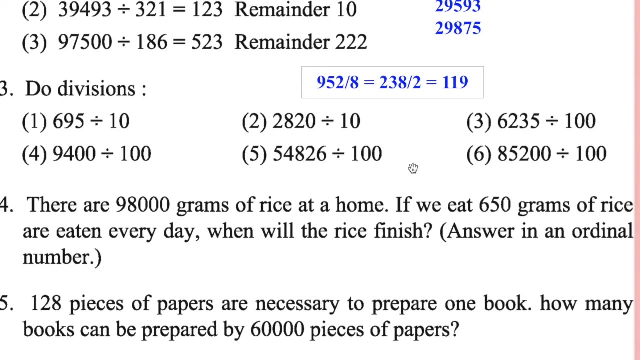 two, nine, one, nineteen numbers. are these okay? one nineteen, clear year. one: nineteen: a person saves money 850 taka in every month. in what month will he is saving exceeds fifty thousand taka? fifty thousand by eight fifty or fifty thousand by eight fifty? the both zeros got cancelled out okay. 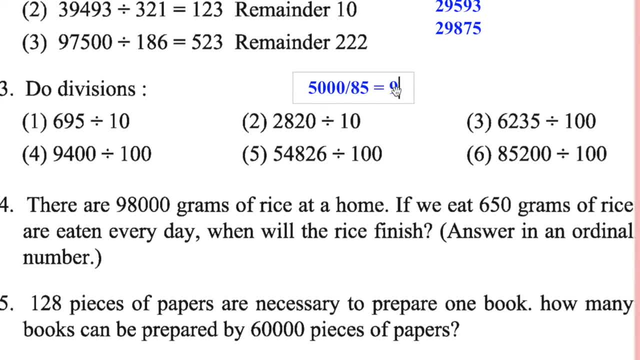 and then the175. alright, we'll go by five. first five, one drop five. uh, five, 7.35, so 17. uh, how many hundreds? 17 or piger 10, 5, 17, forge ł 40, 28 or 58, 155, zack 45Fish. 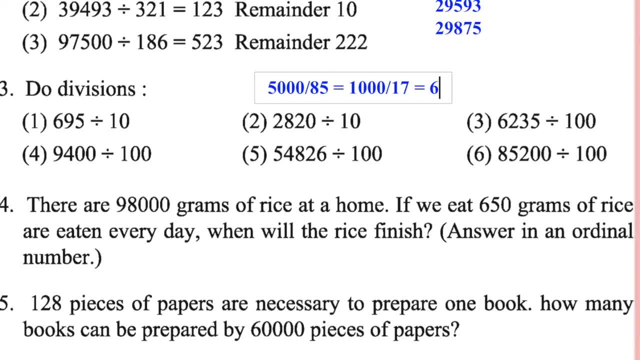 17.6, 17, 5ja 5, 7ja 35,, 5, 3, 85, 17, 6ja 6, 7ja 42,, 2, 4, 1, 0, 2, so 5ja 85,, 85 means. 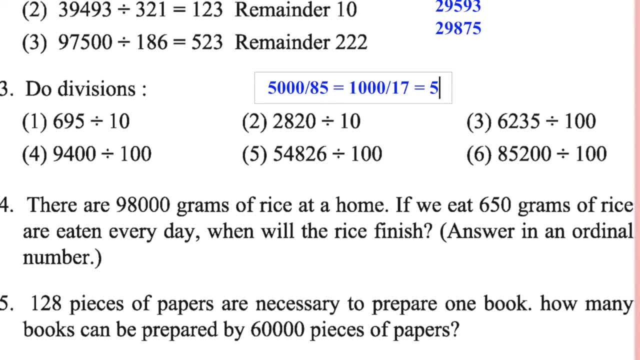 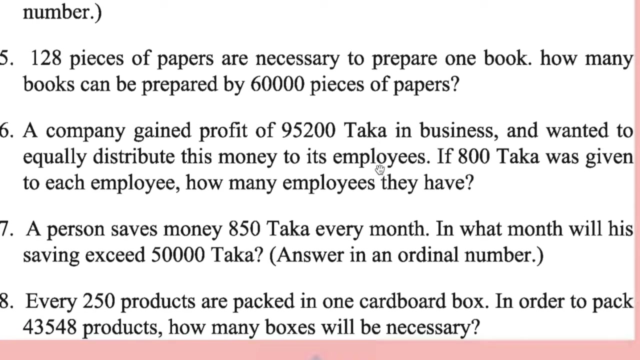 15 will be the remainder, so 150,. 150 means 17,, 7ja 119, 17, 8ja 129 plus 7, 129, 136, um 136, 136 plus 17, that will be more than 150. so 59th month. okay, 136 means 14, so 59th month.